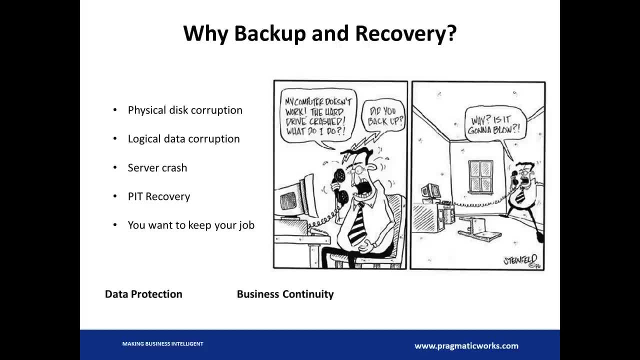 it got approved. change control approved it. The thing is the people approving it don't know T-SQL so they didn't actually look at the syntax of the script. but it was actually a delete on the master table without a where clause, So once that was ran, the entire app. 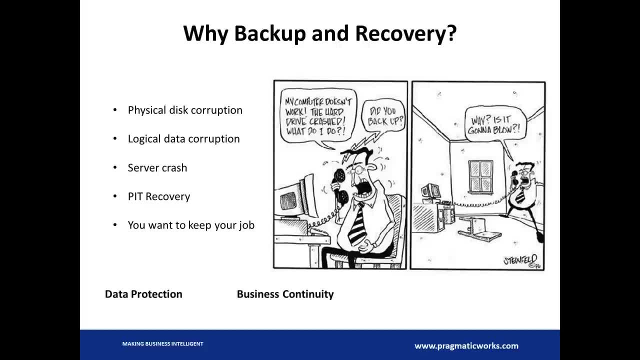 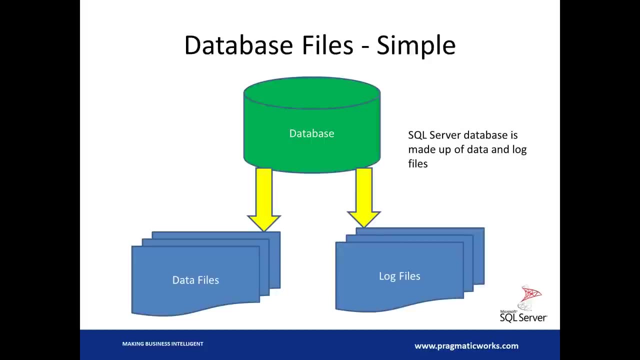 was down. it was down for over an hour just trying to recover from that data loss. So these are things to think about as you're designing your plan. So let's talk about what comprises a SQL Server database. In its simplest form, it's made: 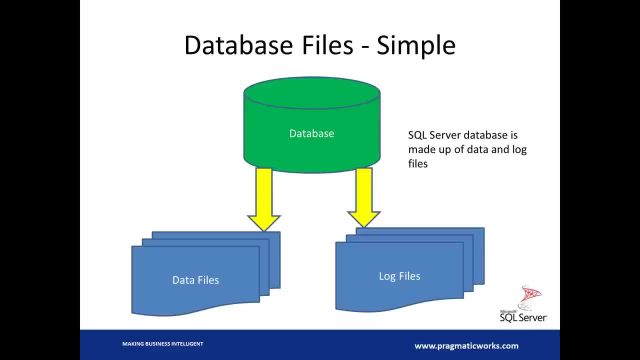 up of data files and log files. It can have multiple data files, it can have multiple log files and it can have multiple log files, even though that's not recommended, because they're written to it in a sequential manner. You know, in its simplest form it's made. 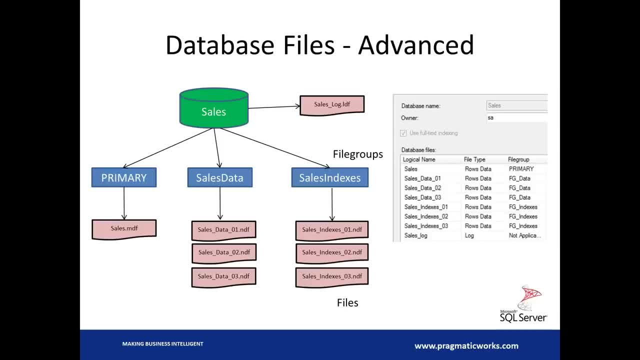 up of data and log files. Now we're going to take a look at a little bit of an advanced form And this is kind of the model I'm going to be using for my demo. So in this picture, you know we have data and log files. You can see the log off to the right up there. 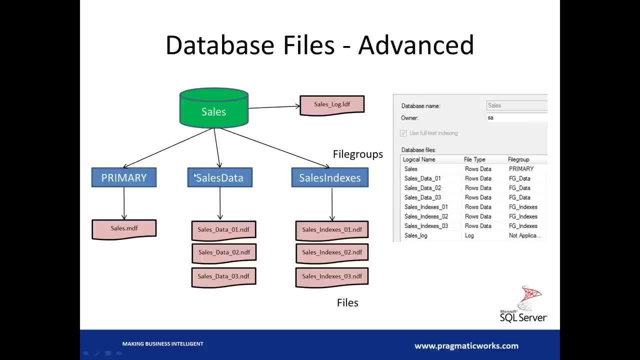 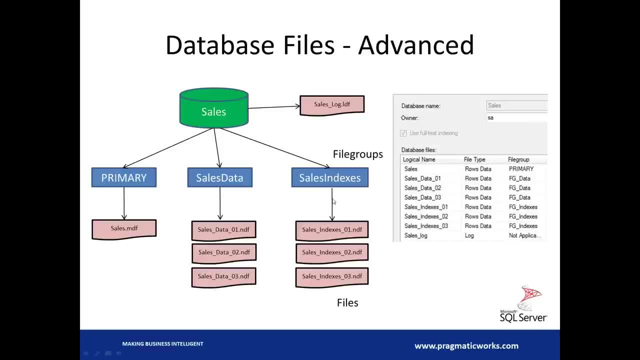 um, well, i might want to put my indexes on on a separate disk in my data. you know to to for performance, for new reasons. you know i want to distribute that io, so so this is a very actually i i call it a best practice is to take advantage of these multiple file groups. um, another example. 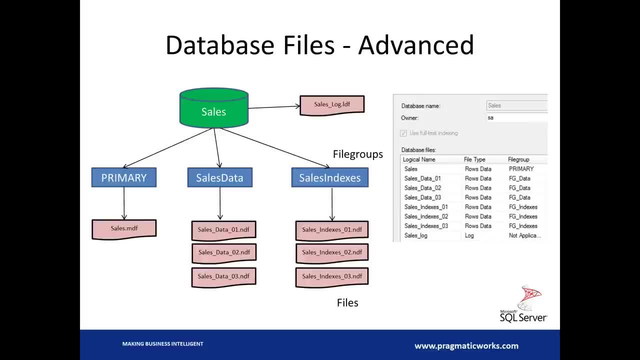 of multiple file groups is you have archive data, you put those in an archive file group and you know it's a point time that could become read only and you can make that file group read only and you can exclude it for maintenance, you can exclude it for backups, stuff like that. so 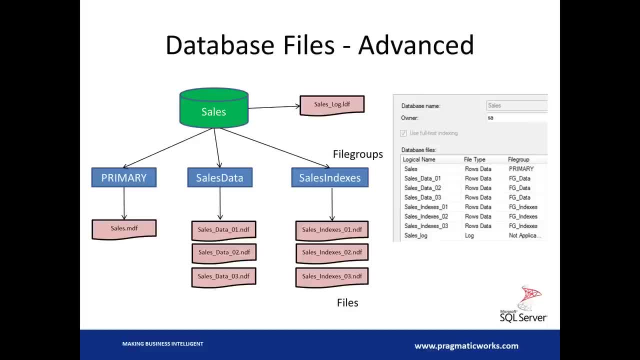 this is a lot of architecture decisions go into, you know, kind of scaling out your database design and and to me, you know, when it comes to being able to restore um and meet those rpos and rtos, that all starts with the architecture of the database itself, um, which is kind of shown in this picture. 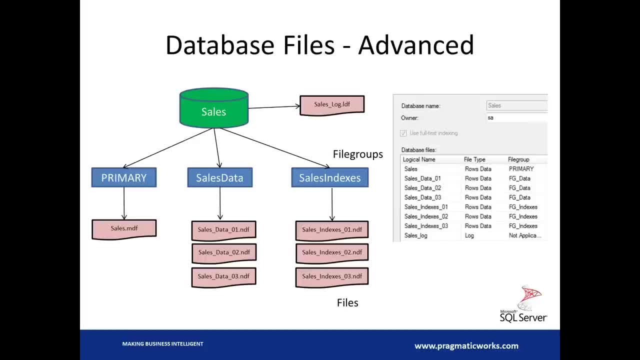 you know we how you want to lay things out. um, another good use i've seen of file groups is, uh, an imaging app. okay, so you know it's got a hundred tables. the database is 200 gig, but 195 gig of that is one table that holds a bunch of. 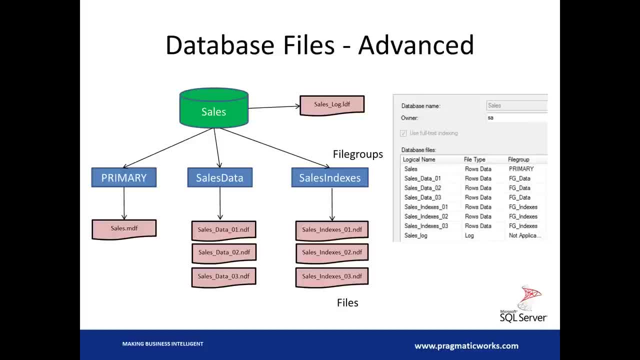 binary images. so if we put those on their own file group then we've only got five gigs of data to manage. you know, for the app to be up, they just wouldn't be able to see their images, you know. so in the event of a disaster i'm only have to recover five, five gigs to bring the app back online. 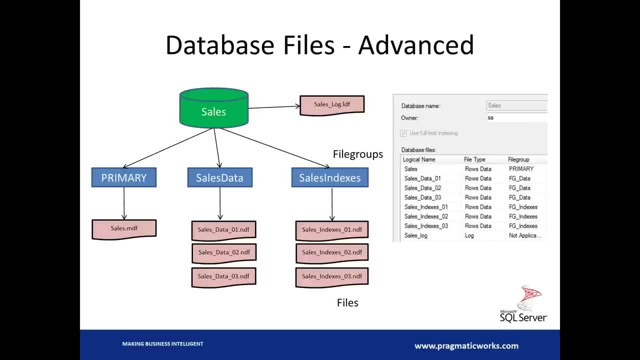 and then we can work on restoring those images. you know, as users are still able to get in and do work, they just wouldn't have access to those images. so, um, those are a few examples of of how you know you can take advantage of these multiple file groups. 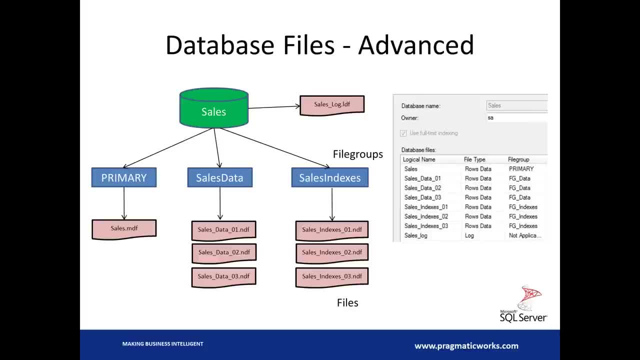 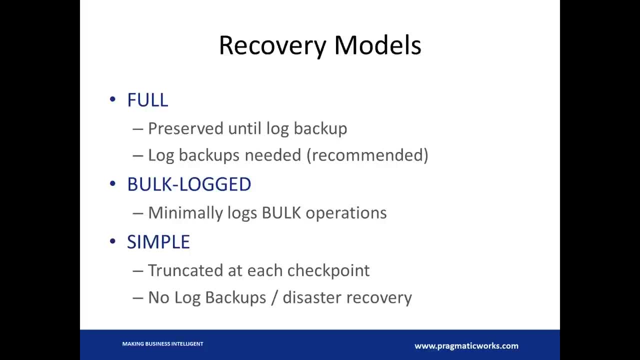 but this is kind of an advanced view of uh database files. so let's talk a little bit about recovery models: um sql server has three different recovery models: full book, locked and simple um. and for those of you who aren't aware, when you create a database in sql server it's going to inherit the properties of the model database by default after you do a. 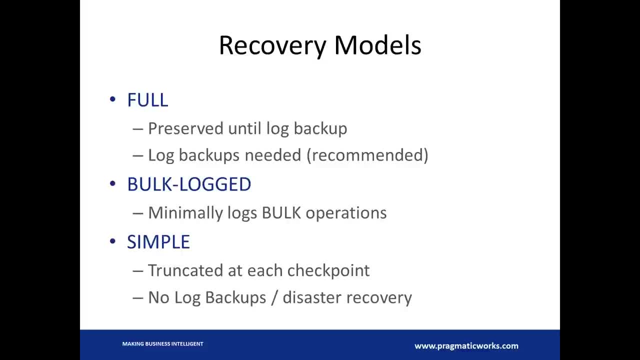 sql server install. the model database is a full recovery mode and i see this all the time: development boxes that have a 150 gig log file and a one gig data file because someone created a database you know not, not taking into account that that model um recovery model. 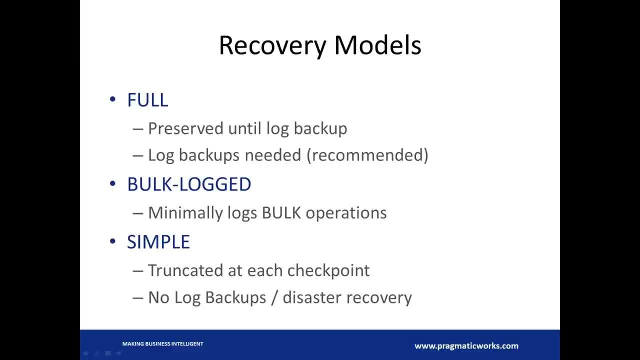 and they haven't been doing any transaction log backup. so basically every transaction ever since that database has been created is just sitting there blowing the log file up, um so that that you know full recovery is basically your log won't be truncated or flushed until you perform a log backup, um to manage the size of your log file for recovery purposes. 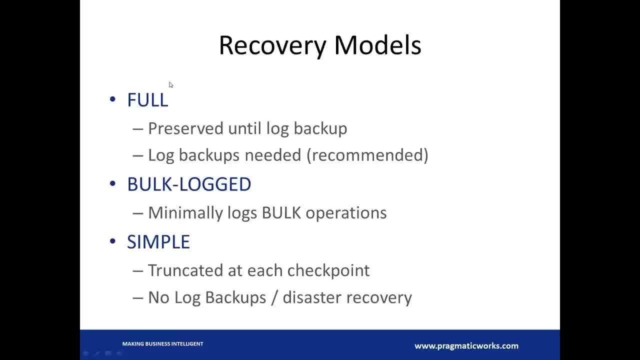 you know, i highly recommend you set up transaction log backups on databases that are in full recovery mode. um, full recovery mode is required for point in time recovery. uh, you know which, which means you're going to be restoring transactions. you're going to be restoring transactions log backups you cannot restore. you can't back up the transaction log in simple recovery mode. 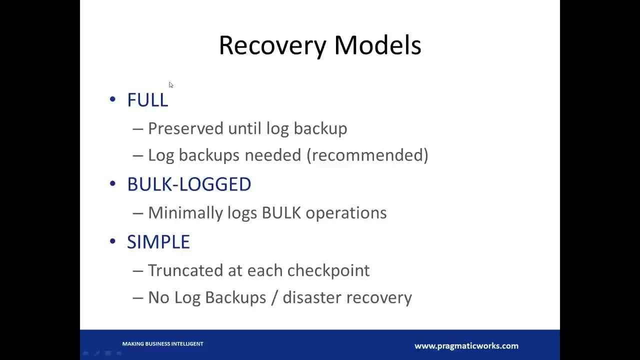 for instance. you know so. so full recovery mode or bulk log recovery mode, either one of those can be used for for point time recovery. the difference in full and bulk logs is bulk operations like insert, bulk bcp. those are minimally logged, you know. they're basically logged at the event occur. 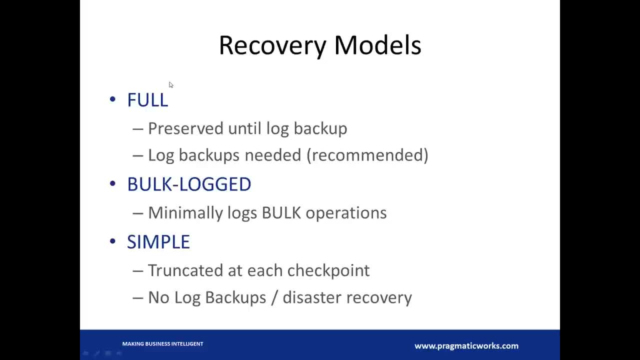 they don't log um the row by row operation. so you know those are the two. i i rarely have seen bulk log used. i i know it has a place in the industry, um, you know, just through my experience i've it's i've never come across a a reason to have to use bulk log. um, but basically. 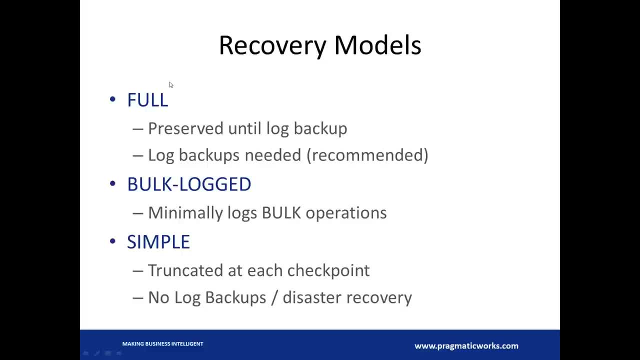 that the difference in it in full is that minimally logged for the bulk operations. i would also recommend log backups on bulk log recovery model, because the log won't get flushed until a log backup is taken. um, now that takes us to simple recovery mode or recovery model. 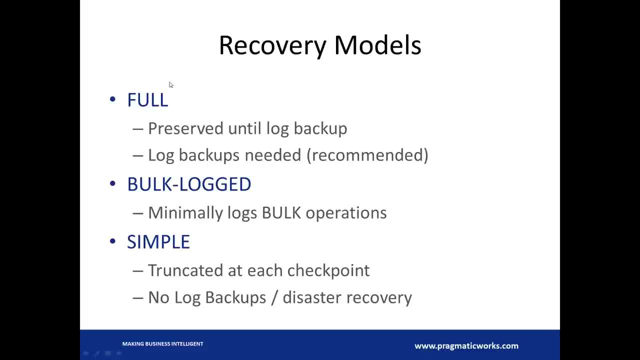 but basically the log is truncated at each checkpoint. you can't take transaction log backups. you don't have the the ability to do point-in-time recovery. that's normally what you're going to see in a. i guess a good business case for that is: i've got a database that gets. 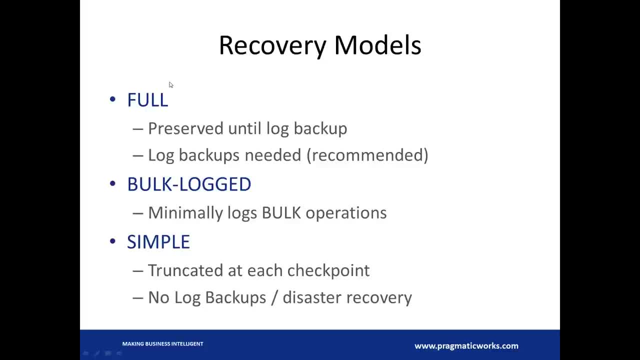 refreshed once a night from another system or from flat files that come in from a client. basically, there's an etl process that runs and it truncates and reloads this database every night at 11 pm. well, at 12 pm i'm going to stick a full backup and i'm done. you know, data's not changing. 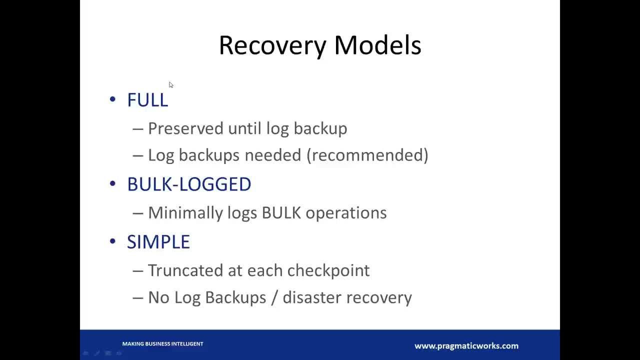 throughout the day, so that that would be a good candidate for simple recovery. another other good candidates would be a development or qa environment, unless you're actually testing the how it affects your app or how it affects the log files, certain functionality within your app, you know you.